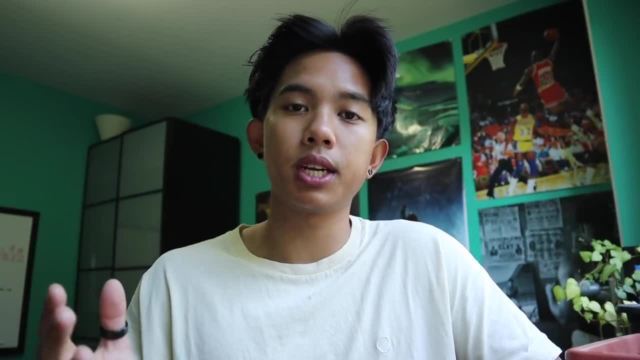 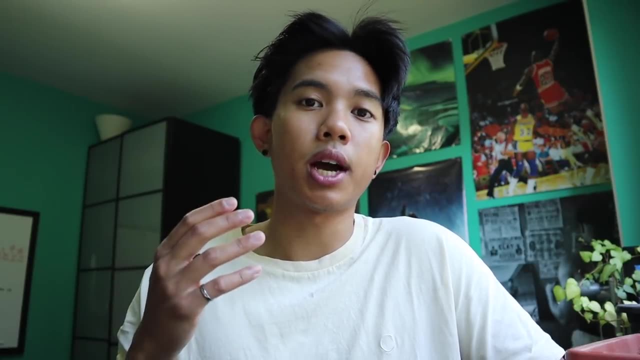 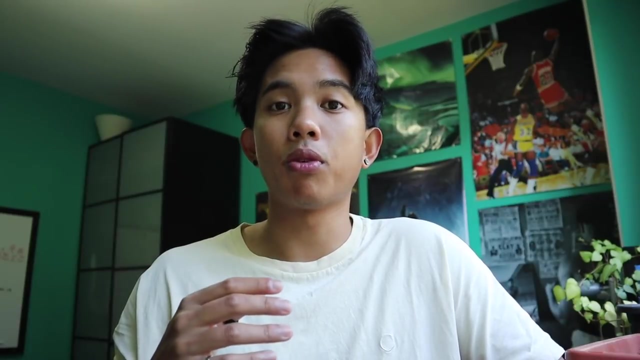 within minutes. all you need to do is drag and drop some blocks, connect some streams together and add some inputs. From that point on, you can set up some sensitivity analyses, some optimization functions to try and increase the efficiency and, more importantly, the profitability of the process. Process simulators are often used before making big changes in your 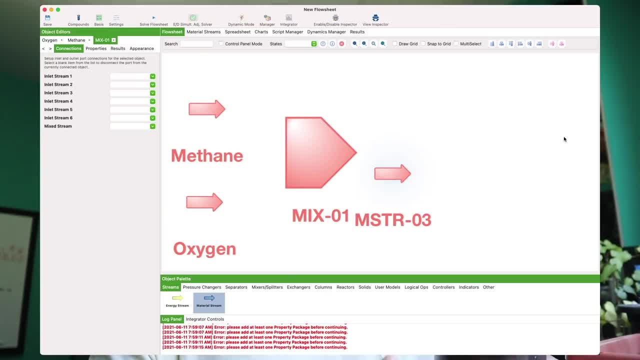 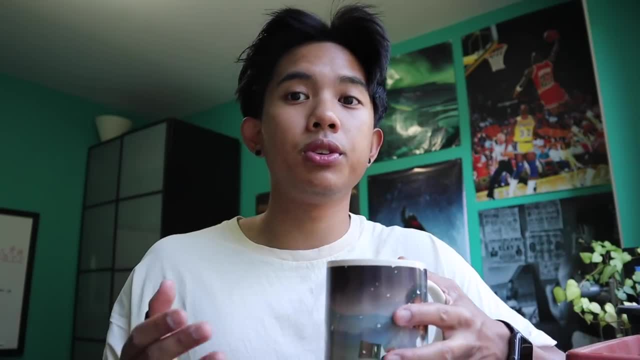 plant to try and predict what would happen. So the thing that I'll be showing you on the screen is called dw sim, and with dw sim you can do process flow sheeting. So one thing you could do as a student to not only improve your proficiency at process flow sheeting but to also maximize your 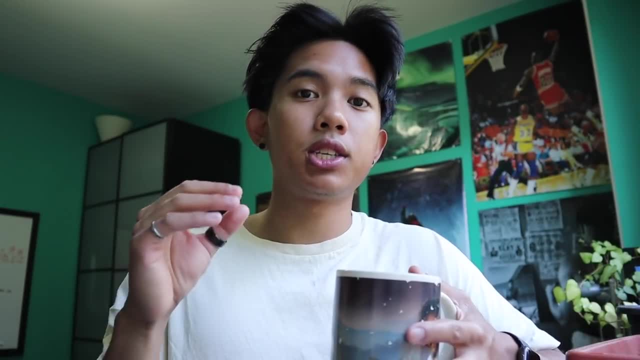 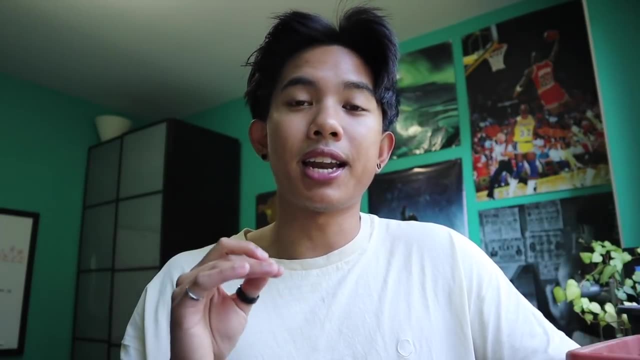 chances of getting into the industry that you want to get into is to look up a research paper. So let's say you want to get into the hydrogen industry and the dominant way that hydrogen is made today is steam methane reforming. About 95% of hydrogen is made by steam methane reforming. 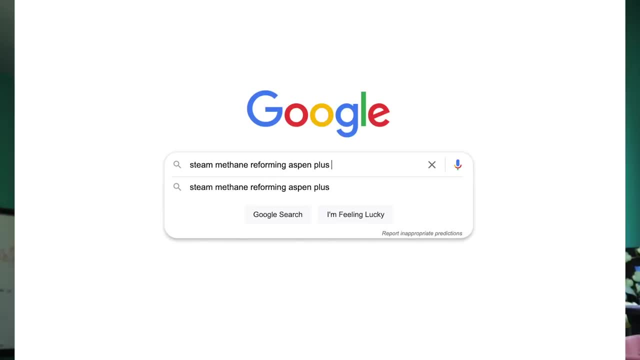 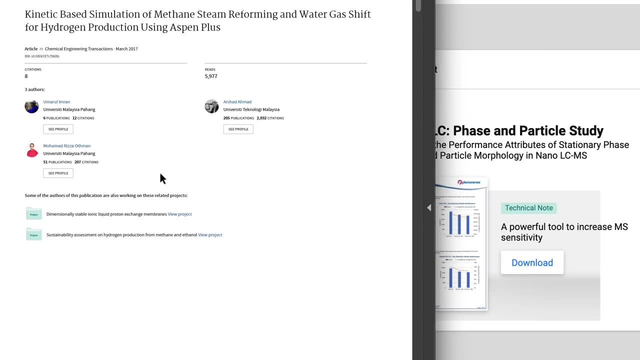 About 95% of hydrogen is made by steam methane reforming, So you could look up a steam methane reforming aspen plus research paper. copy the entire flow sheet. they will give you the entire flow sheet as well as some of the inputs and if there's anything not, 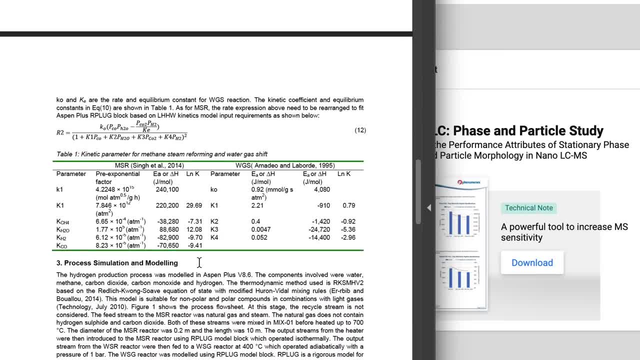 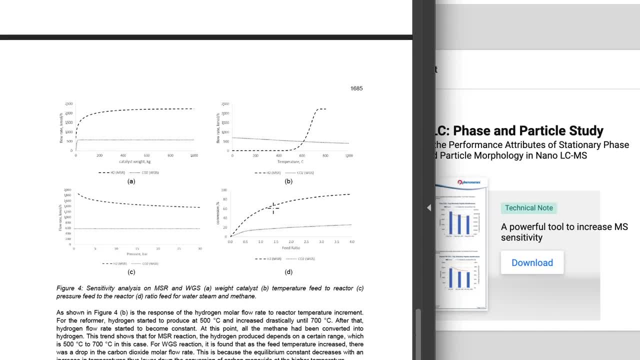 provided you could just plug in some numbers and guess, do some sensitivity analyses on it, write an optimization function and just play around with the software. and once you do this and create this mini project of your own, you can put this on your resume and when you're applying for hydrogen cut. 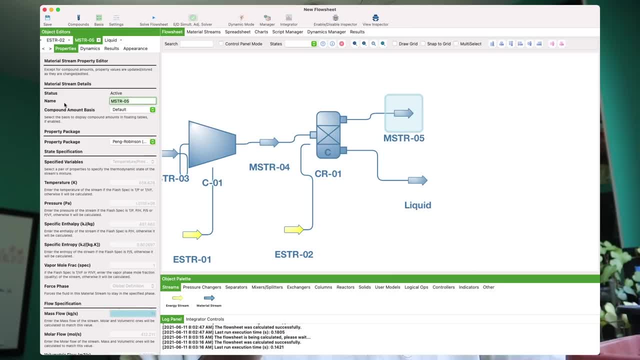 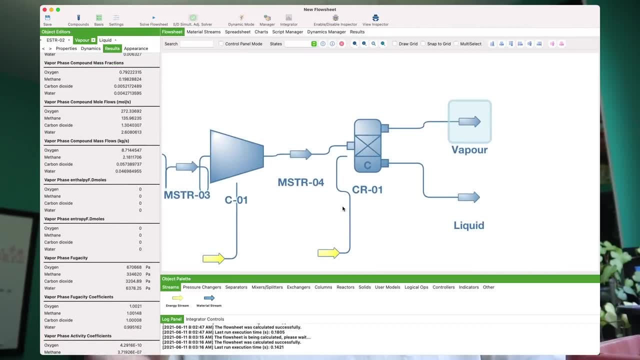 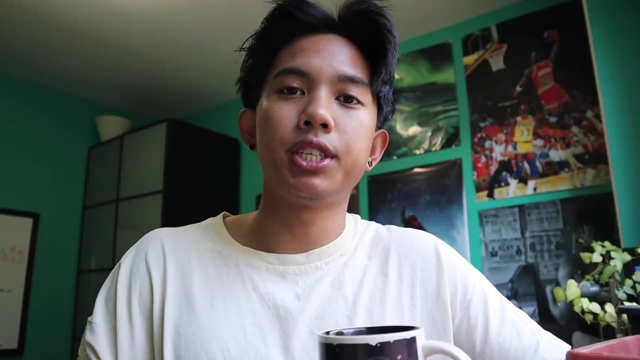 companies. this is going to look really, really good, because not only have you increased your proficiency at a relevant skill- aspen plus through the use of dw sim- you've also created a specific project that is going to help you get the job. so the second important skill of chemical engineering: 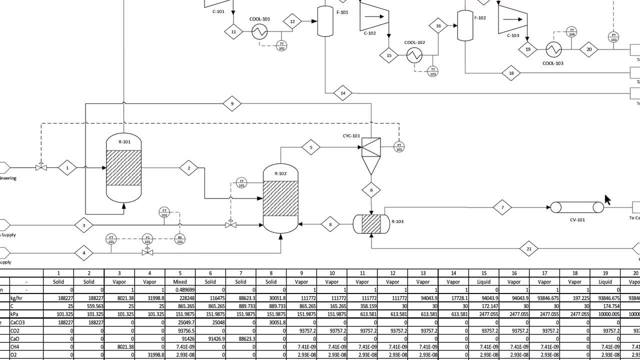 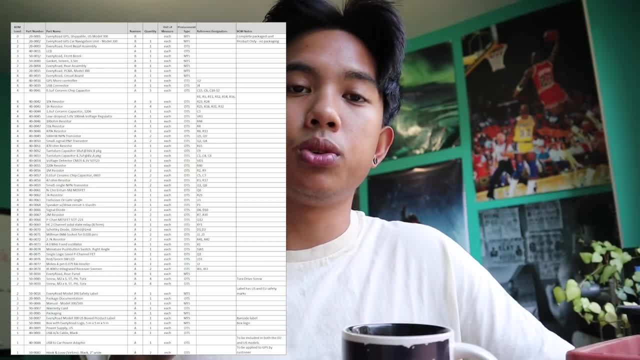 is the engineering documentation i'll call it. this includes everything from process flow sheets, or pfds, to piping and instrumentation diagrams, or pnids, to build materials, which is a bomb, to facility layouts, and there's probably a bunch of other ones that I missed. 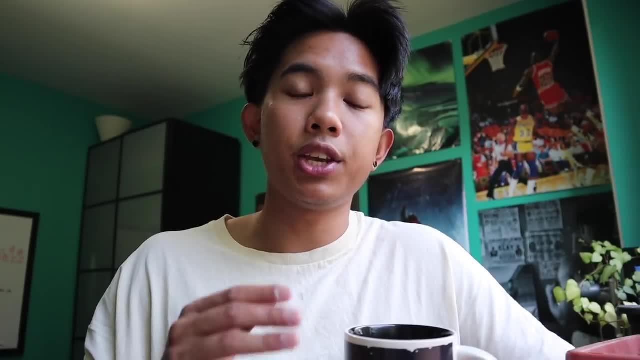 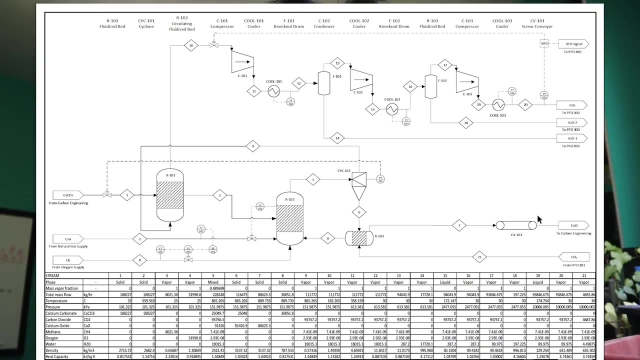 These are all a really, really crucial part of plant design and you'll likely get a chance to learn how it works during your capstone project in your final year. So PFDs are the temperature, pressure composition data of every single stream in the process. 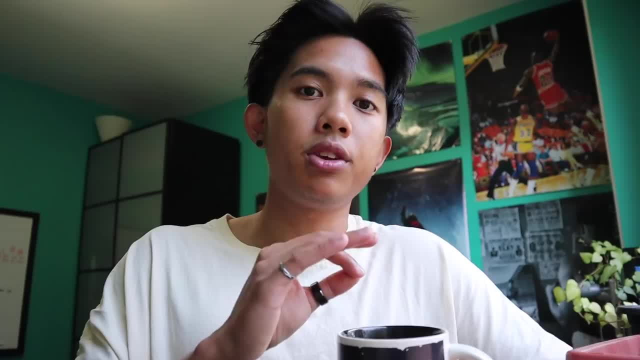 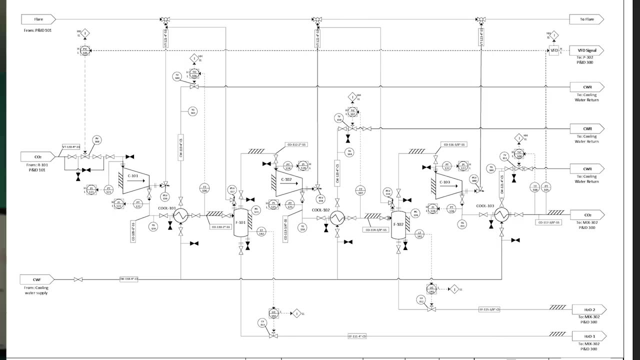 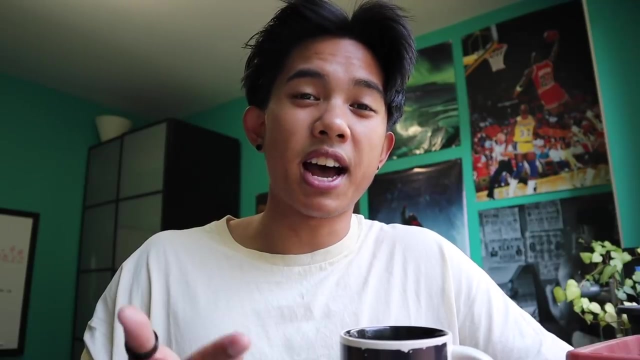 and you can usually get this data from Aspen Plus. Then you go into the lower level details of a P&ID where you talk about the actual control systems that are used to maintain those temperatures and pressures that you specified. It also includes piping sizes, valves, 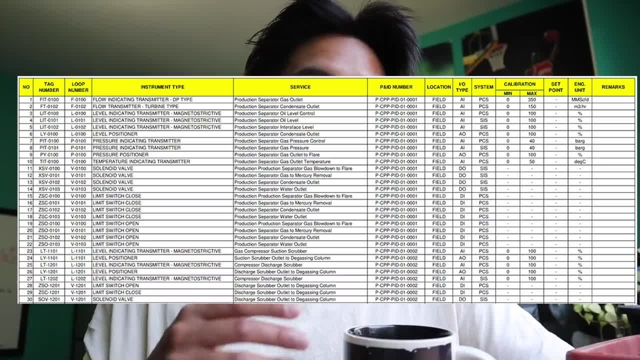 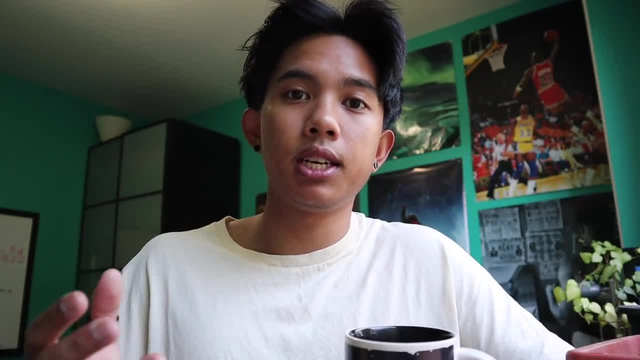 and other good stuff that you need to make the plant run. In the P&ID you can build IO lists, which are input and output lists. You can build your list of equipment that you're actually going to need. The bill of materials is basically a grocery list. 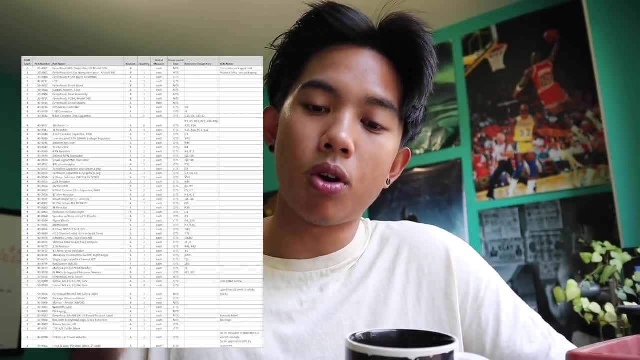 of stuff that you need to buy for the plant and it can give you a overall cost that is needed to fund that. So if you're going to build a P&ID, you're going to have to spend a lot of money on the project. 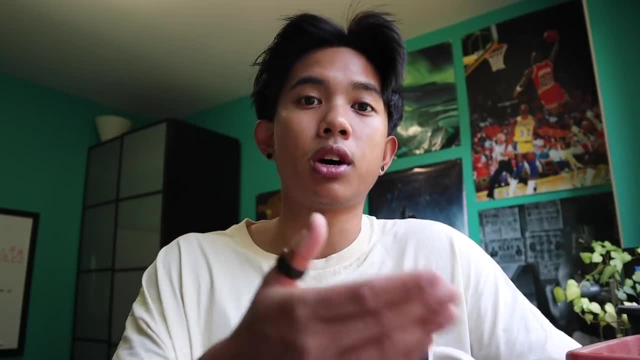 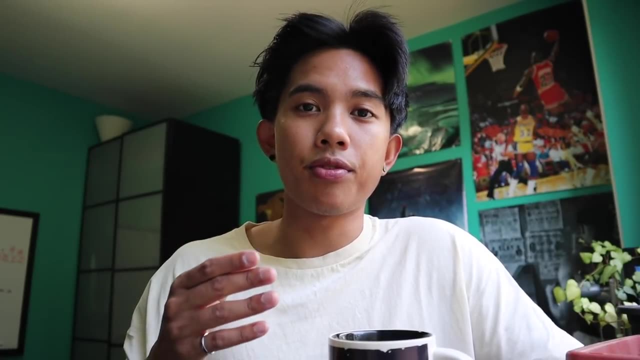 Each of these documents is important for chemical engineers, not only to understand but to be able to mark up, to talk over or to make one from scratch. Unfortunately, these skills aren't really taught that well in school, and the way that I've actually built up these skills- is through internships, And I know that's not really helpful. How do I get the internship if I don't have the skill? yet If you aren't able to land an internship, then being a part of an engineering design team can be a big challenge. 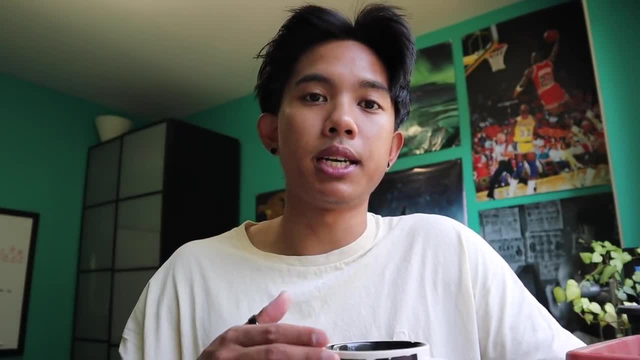 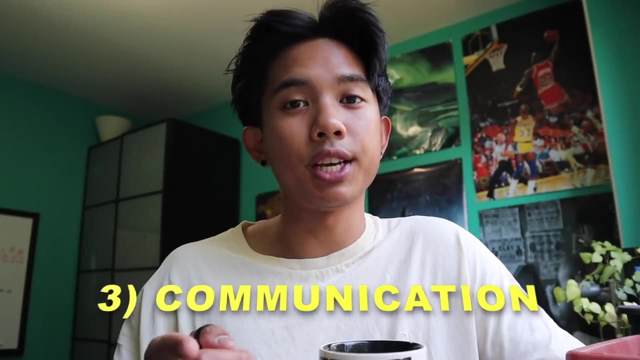 So I'm going to go back to maybe one or two of these pieces of documentation. At least, when I was part of a design team, I did look at a bunch of PFDs and was starting to look at P&IDs before I left. 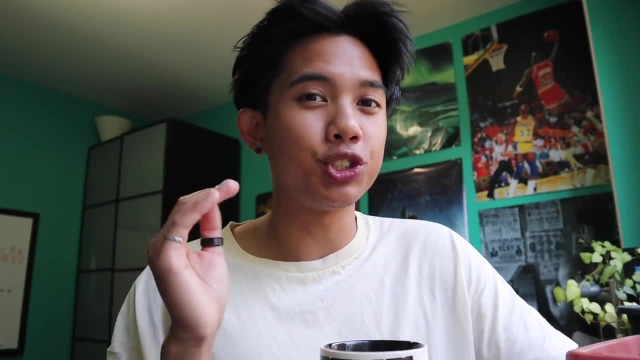 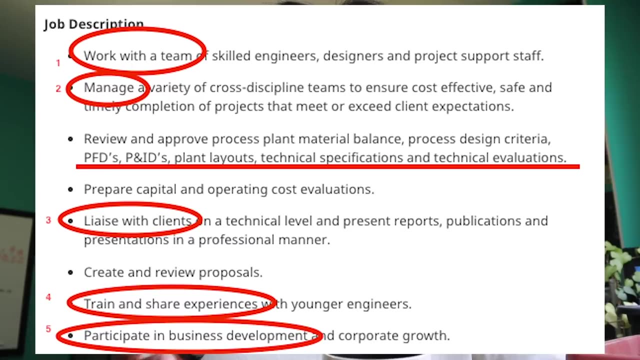 So the third skill is communication, and although it sounds super cheesy, please don't click out of the video. I mean, if you look at this job description that I pulled from the internet, five out of like the 10 job responsibilities involves some aspect of communication. 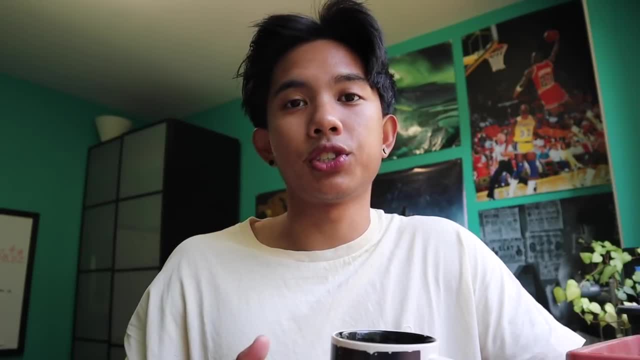 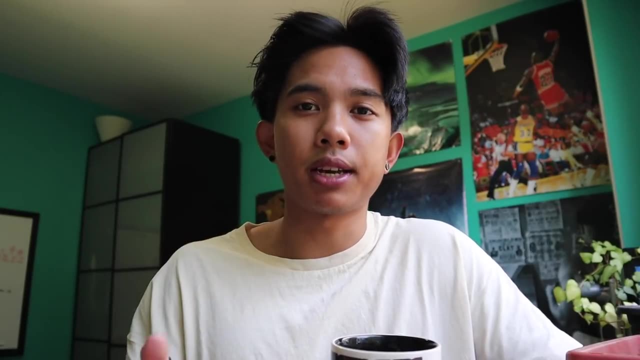 Although being a good communicator is a soft skill, work is never done in isolation. As a chemical engineer, you might have to talk to mechanical engineers, you might have to talk to electrical engineers, the project manager, and it's rare that you'll ever just do one project. 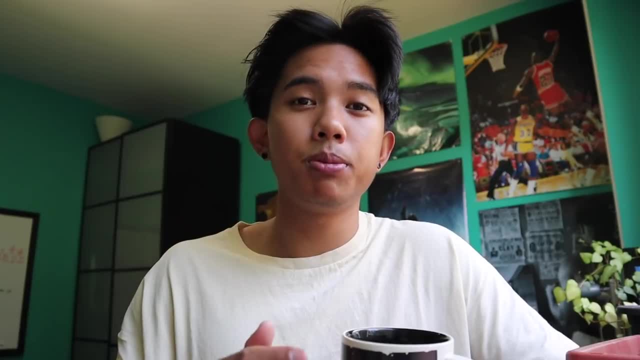 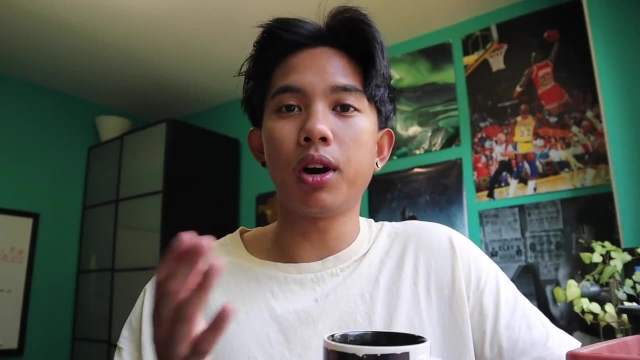 on your own for months on end, right? So you need to be able to communicate with other people to get them what they need and also ask for things that you need to get your job done. So we all know that you should improve your communication skills. 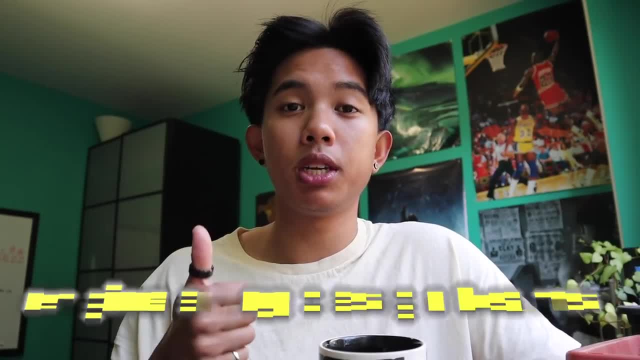 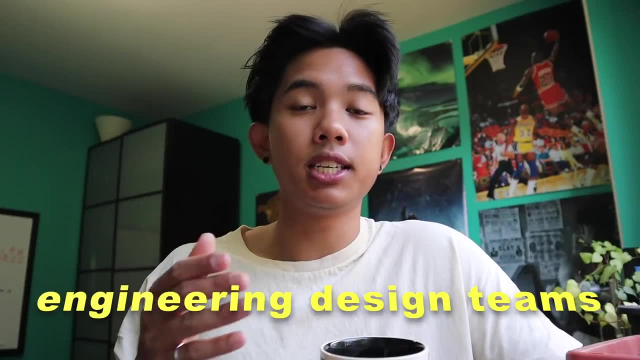 but how do you actually do this in real life? My number one piece of advice would be to join a design team. I found that when I have told employers that I was part of design teams, they liked the fact that in design teams you work with different engineering disciplines. 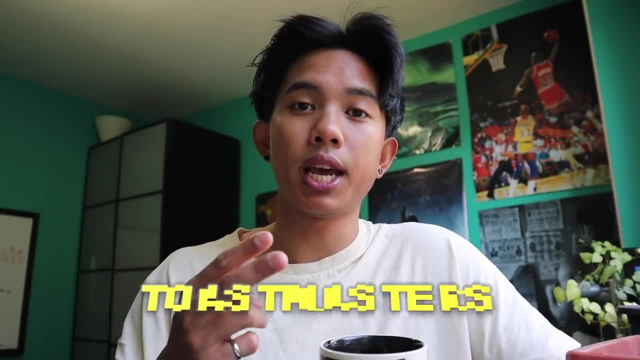 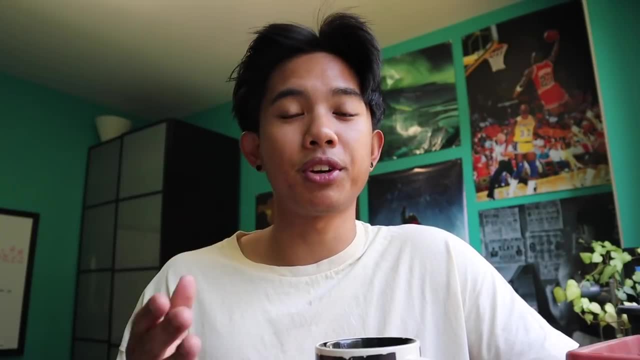 just like you'll be doing in the workplace. The second piece of advice would be to join a public speaking club, such as Toastmasters, where you actually learn how to deliver speeches that captivate audiences. And my third tip- and I've gotten this from actual working engineers- 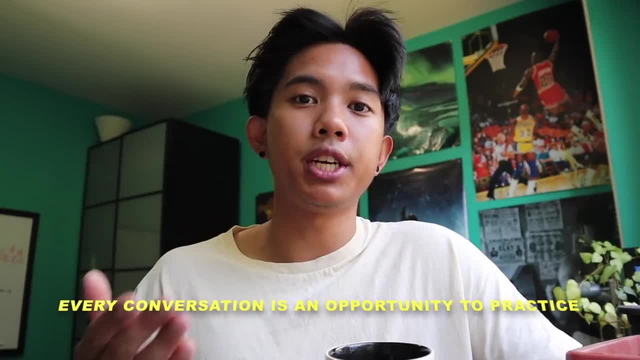 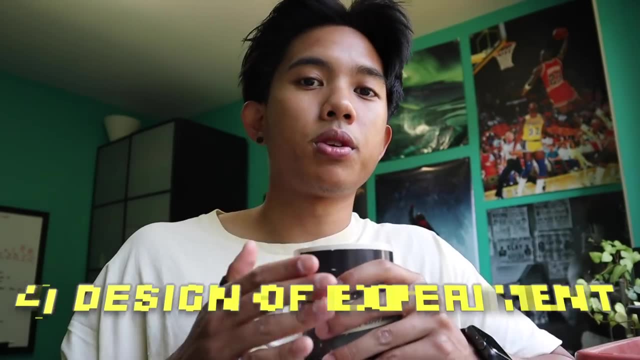 who have given me advice on how to be a better communicator is to just be more present in your daily conversations, Whether you're talking to your friends, talking to your family, make sure that you try your best to be a better communicator. So the fourth skill is design of experiment. 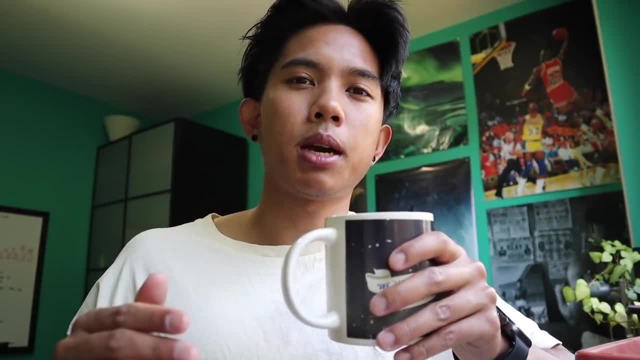 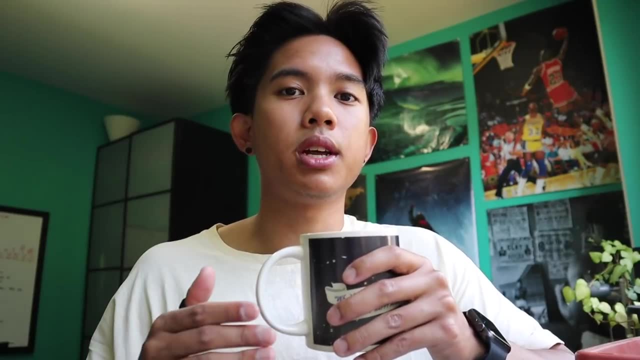 It's a skill that I've seen commonly in more R&D type roles- stuff that I've seen in the pharmaceutical and semiconductor industries. So, although simulators like Aspen Plus are really good at predicting your final product, at some point you're gonna wanna verify that. 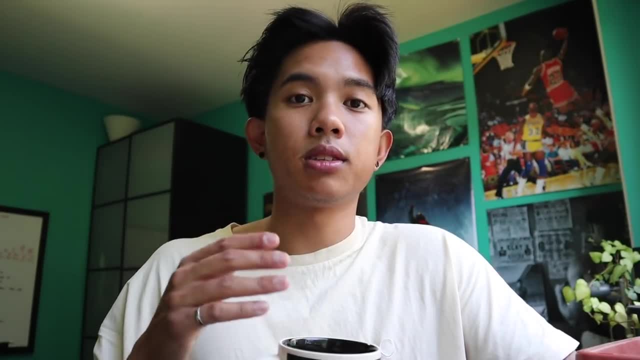 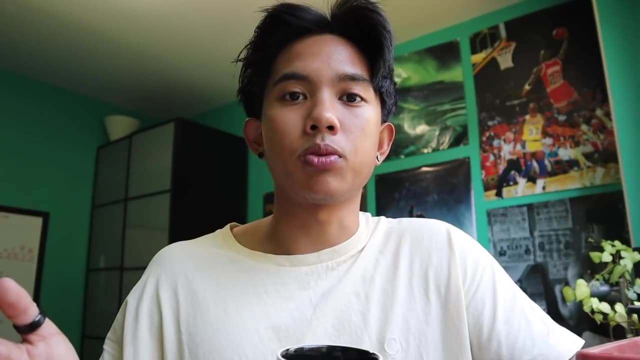 by designing an experiment. As a process engineer. you need to understand statistical data analysis at some level to be able to create experiments analyze the results. In undergrad, the thing that I always dreaded was doing the error analysis in our lab And looking back at it now. 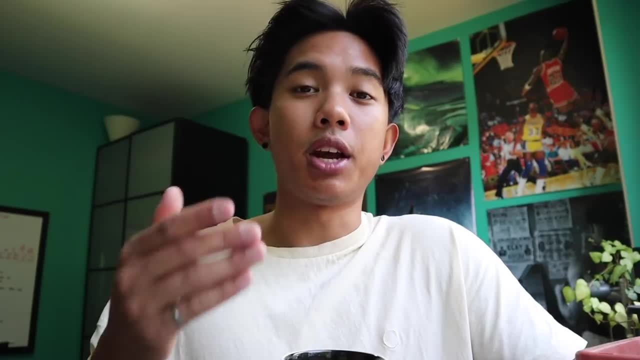 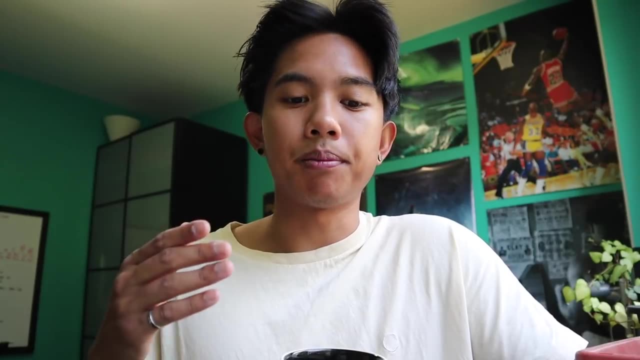 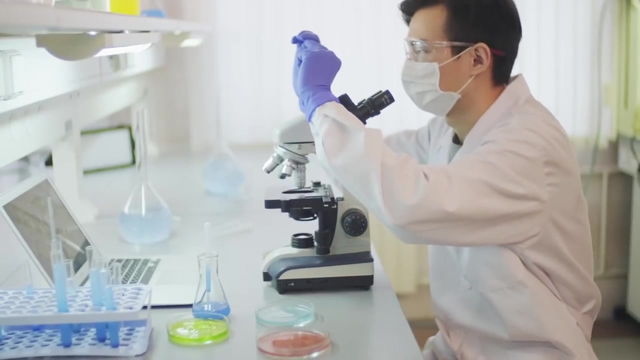 it was actually really, really important because when you communicate a number in the workplace, oftentimes people want to know how confident you are in that number, And error bars give us a pretty good indication of how confident you are in that answer. In my last year of chemical engineering, 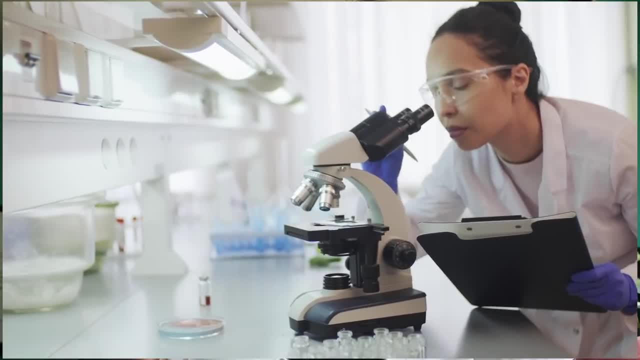 our lab project was completely self-guided, So that's a huge opportunity to be able to do that. So that's a huge opportunity to be able to do that. So that's a huge opportunity to be able to do that And that's a huge opportunity to really build. 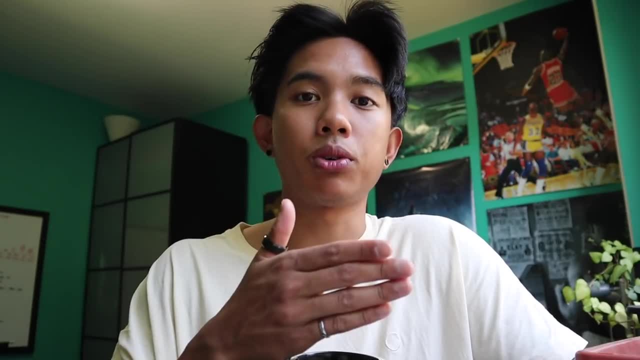 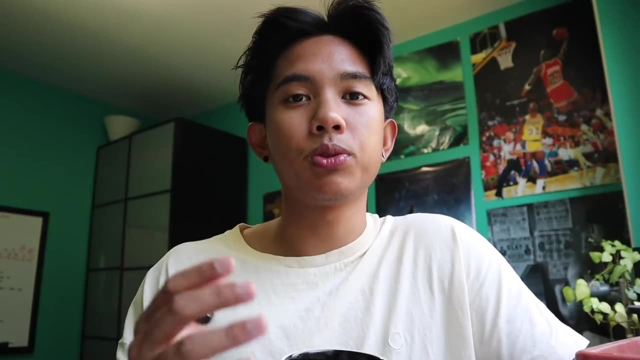 your design of experiment skills, where you actually have to plan out what tests you'll be running And then you have to, from that kind of reverse engineer the type of analysis you're gonna do. So that's really helpful and can really build your design of experiment skills. 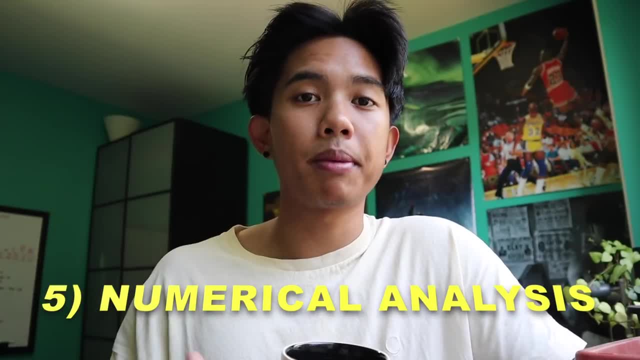 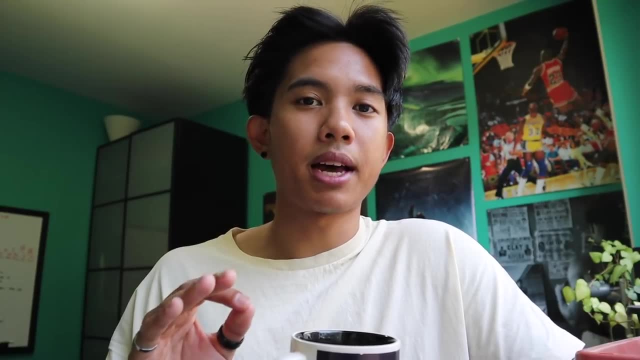 So the fifth skill is mathematical modeling, or coding, or programming, or whatever you wanna call it. So, while the four skills I mentioned at the start are definitely the most important for chemical engineers, having mathematical modeling or numerical analysis as a skill can be your secret weapon. 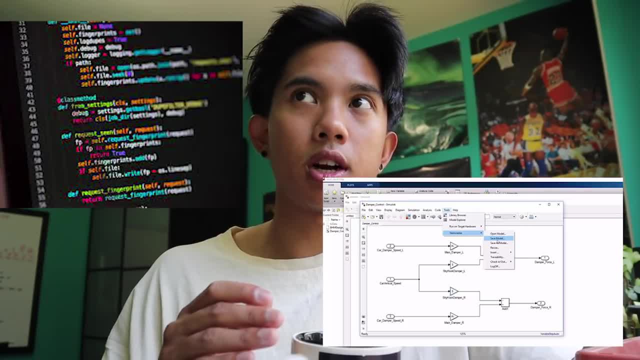 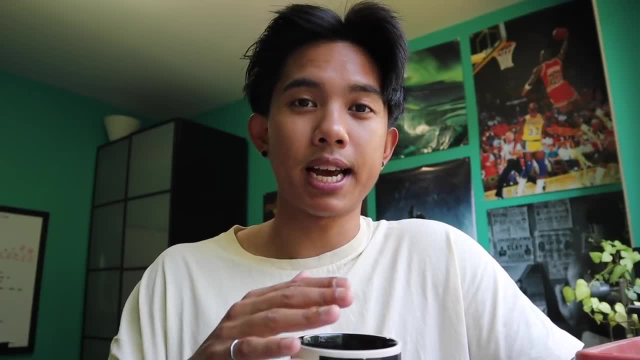 While knowing how to code is not currently a job requirement, it's starting to pop up a lot more in different job applications. For example, I know a couple of people working at a renewable energy software company right now, and all they're doing is coding every day.